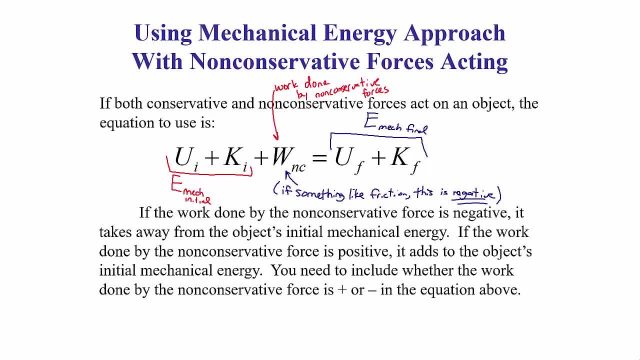 by the non-conservative force is negative, it's taking away from the object's initial mechanical energy, and so if that work is positive, it is adding to the object's initial mechanical energy, and in that equation we include whether the work done by the non-conservative force is positive or 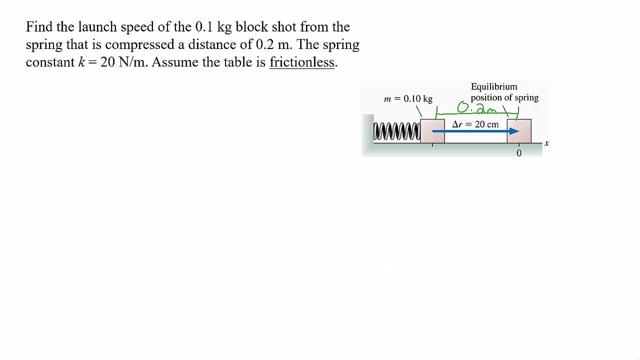 negative. so to understand this, let's look at the situation of a box that's pushed up against a spring. first, we're going to look at the case where we have conservation of mechanical energy, where we have no non-conservative forces, and we have non-conservative forces and we have 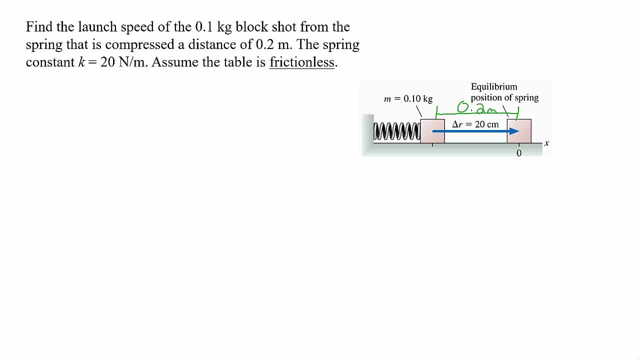 no friction acting, and so there are no non-conservative forces doing work. this 0.1 kilogram block is pushed up against a spring and it compresses the spring a distance of 0.2 meters, and the spring has a spring constant of 20 Newtons per. 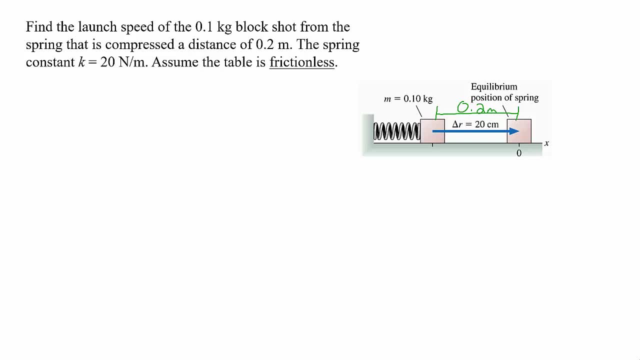 meter and we want to figure out what is the launch speed of the block as it's shot from the spring. potential energy stored in a spring is 1 half K. X squared K is the spring constant. X is the spring constant. X is the spring constant, X is. 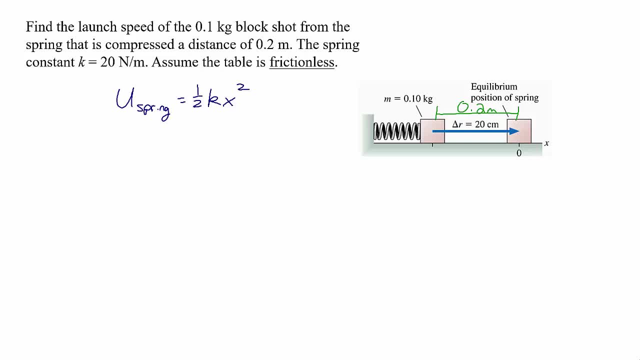 how far we stretch or compress the spring from its equilibrium or unstretched position. so conservation of energy says that the potential energy at point a plus the kinetic energy at point a equals the potential energy at point B plus the kinetic energy at point B. I'm gonna call point a the spot where the 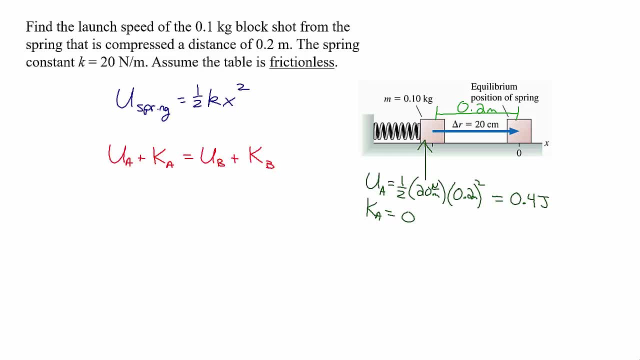 spring is compressed where we have energy stored in the spring. the potential energy stored in the spring is 1 half kx squared, 1 half times 20 Newtons per meter. per times 0.2 meters squared, The potential energy stored in the spring is 0.4 joules and that box. 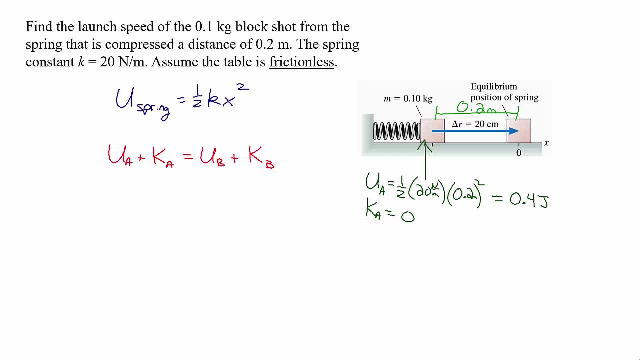 is starting from rest, so the kinetic energy at the beginning is zero. Now the spring pushes the box to the right and it reaches that position where the spring is not compressed anymore and the box is shooting off of the spring. So because the spring is not compressed anymore, the spring 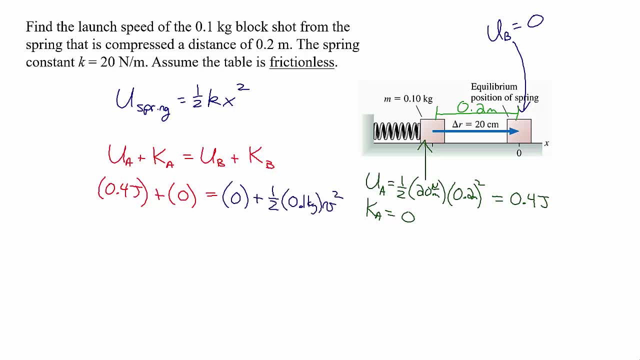 potential energy at the end is zero and the kinetic energy is one half mv squared. One half times 0.1 kilograms times the speed squared. And so, looking at this, we have everything in our conservation of energy equation that we need to be able to solve for the speed We get, that the 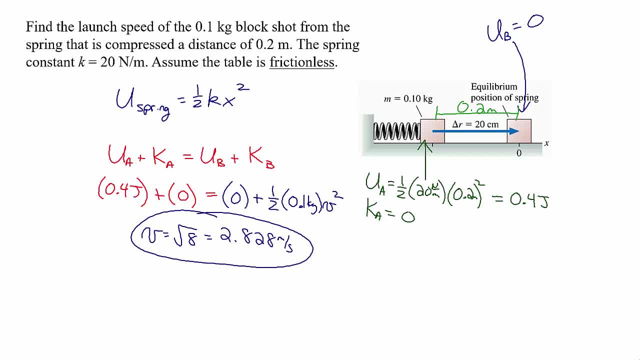 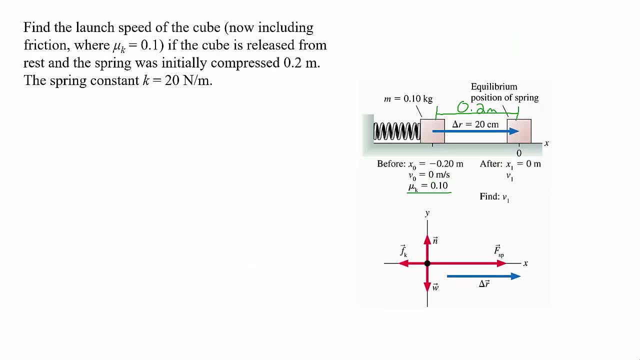 speed as it leaves, the spring is 2.828 meters per second. But now what if the table was not frictionless? What if the coefficient of kinetic friction between the block and the table was 0.1?? And so it's the same situation, where the box compresses the spring by 0.2 meters. 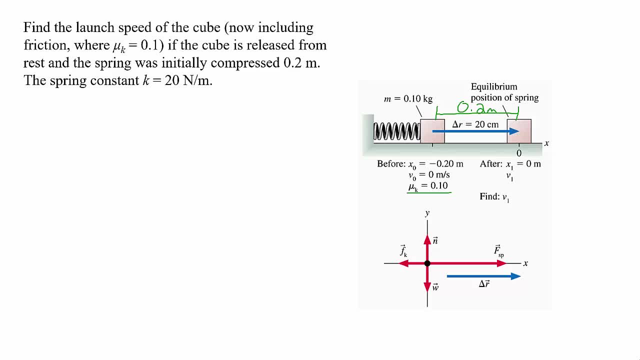 and the spring shoots the box to the right. We want to find the speed of the box when it leaves this spring. Our conservation of energy equation says that the initial potential energy plus the initial kinetic energy, plus the work done by the non-conservative forces equals the final potential. 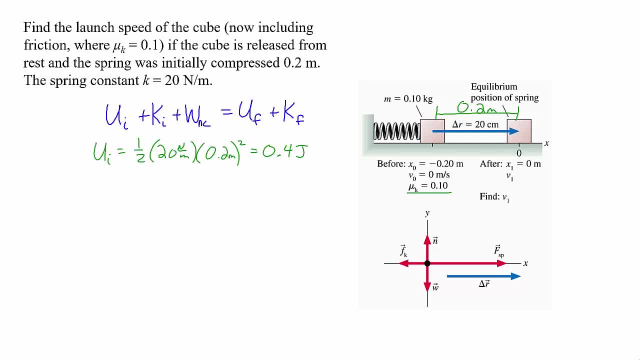 energy plus the final kinetic energy. At the beginning it's still the 0.4 joules of potential energy stored in the spring, And again the box is starting from rest, so the initial kinetic energy is zero. So then we have to find the work done by the force of friction. 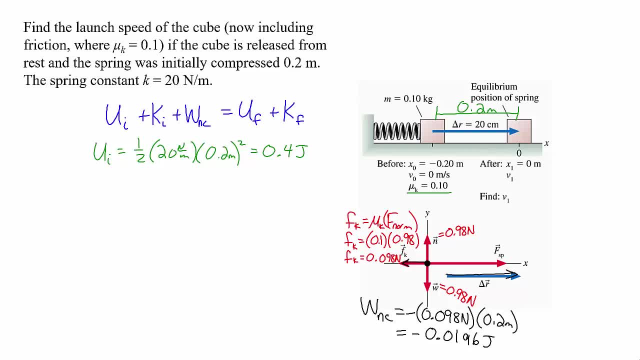 Again in that equation: WNC, that's the work done by the non-conservative force. So we're looking for the work done by the force of friction. The force of friction is the coefficient of kinetic friction times the normal force, And here the normal force is going to equal the weight of the block. The weight of the block is 0.98. 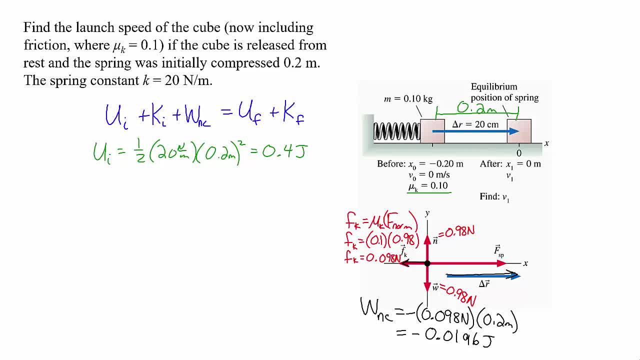 newtons, 0.1 kilograms times 9.8 meters per second squared. Because there are no other vertical forces acting, the normal force has to equal that force of gravity. So the force of friction is the coefficient of kinetic friction, 0.1 times the normal force, 0.98 newtons, And the force of friction is 0.098 newtons. 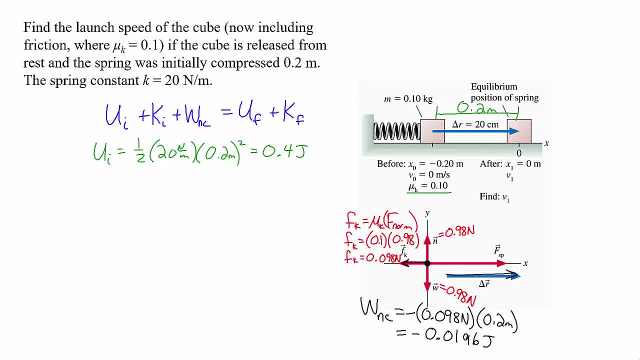 And so the work done by that force of friction is negative. because the force of friction is acting to the left but the displacement of the object is to the right. So if a force is in the opposite direction that the object is moving, that force does negative work. So the work done by friction 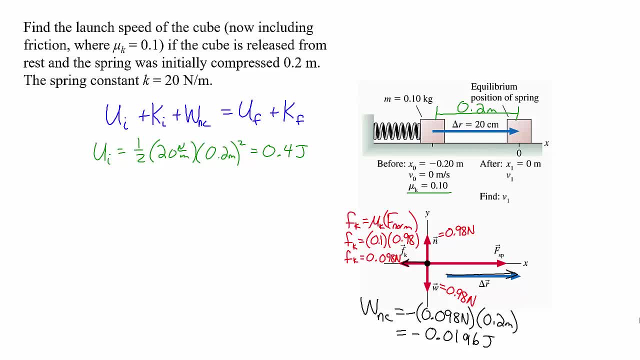 is negative. the force 0.098 newtons times the distance of 0.2 meters. So the work done by friction is negative: 0.0196 joules. We need to include that negative sign when we include the work done by the. 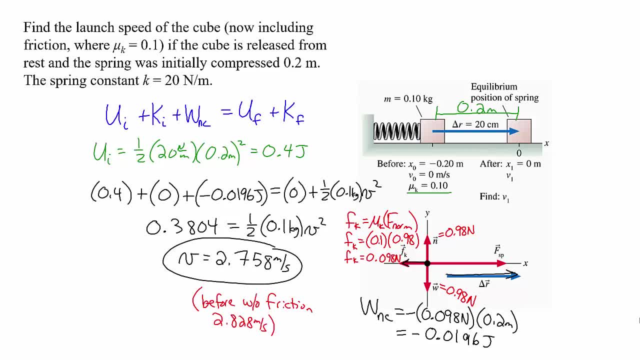 non-conservative force in our equation. So the initial potential energy of 0.4 joules plus the initial kinetic energy of 0 joules, plus the work done by the non-conservative force of friction, negative 0.0196 joules, equals the final potential energy of 0 plus the final kinetic energy. 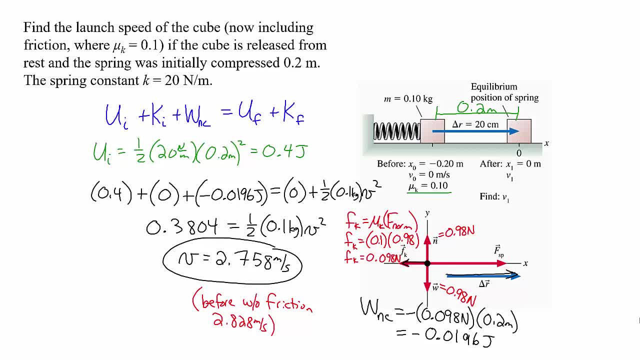 which is 1 half times 0.1 kilograms times v squared. We started with 0.4 joules of energy, Friction took away 0.0196 joules, So we have 0.3804 joules. That's what this whole left-hand. 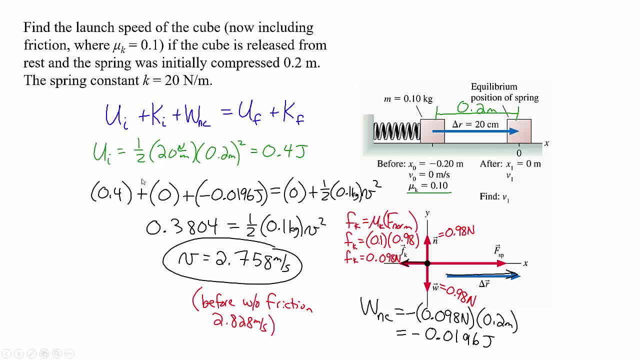 side is telling us: We have a certain amount of mechanical energy that we started with, and then this is how much it changed by, how much it increased by or, in this case, how much it decreased by. So at the end we only have 0.3804 joules of mechanical energy. All of that mechanical energy is kinetic energy. 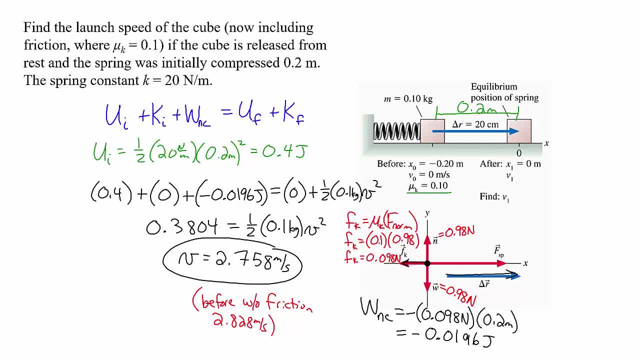 in this case. So 0.3804 joules equals 1 half times 0.1 kilograms times v squared, which gives us a speed of 2.758 meters per second. Again, in the previous case, when there was no friction, the speed was 2.828 meters per second. Here, because of the force of. 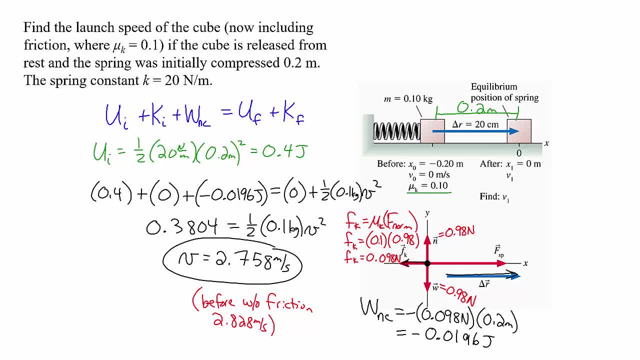 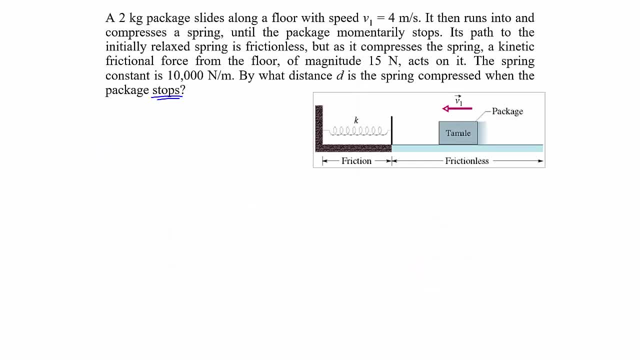 friction. the block left the spring With a slightly smaller speed. friction took away some of the energy that the spring was giving to the block. Here's a slightly different version. I have a 2 kilogram box that's sliding along the floor with an initial speed of 4 meters per second and it's sliding along a frictionless 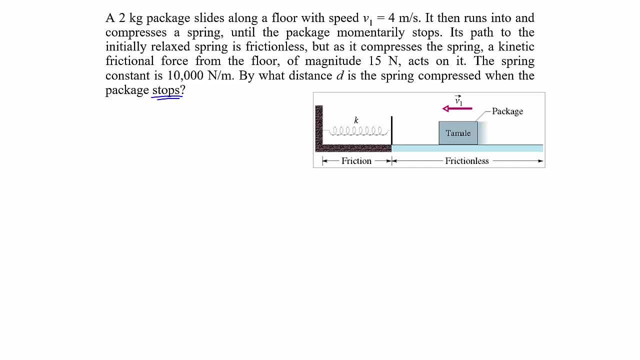 surface initially, and it hits a spring and it compresses the spring a certain distance, Everywhere up until it reaches the spring, is frictionless. but as it compresses the spring, there's a force that's going to hit the spring and it's going to compress the spring a certain distance. 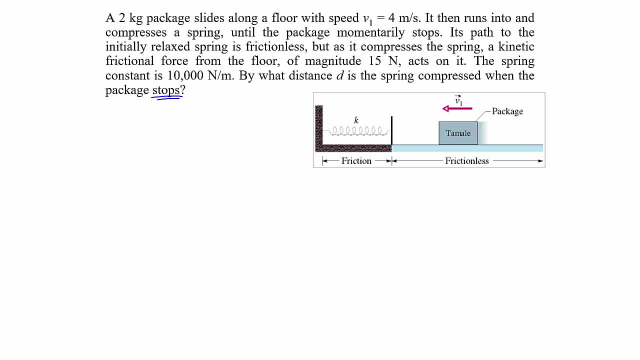 Here's a force of kinetic friction that has a magnitude of 15 newtons acting on the box. Again, instead of giving us the coefficient of friction and the normal force, they're just telling us the force of friction is 15 newtons, But if the box is sliding to the left, that force 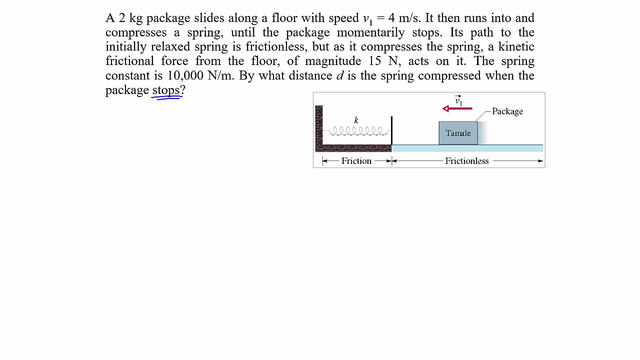 of friction is going to be acting to the right, opposing the motion of the object. The spring constant K is 10,000 newtons per meter and we want to figure out how far is the spring compressed when the box stops. So our more general conservation of energy equation says that the initial potential 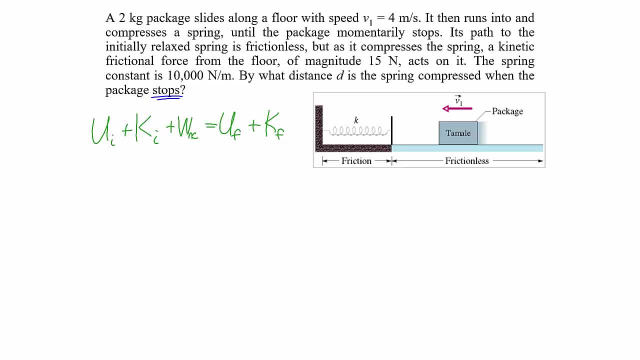 energy plus the initial kinetic energy, plus the work done by the non-conservative forces equals the final potential energy plus the final kinetic energy At the beginning. the spring is not compressed, so there's no potential energy stored in the spring. The kinetic energy is 1 half mv. 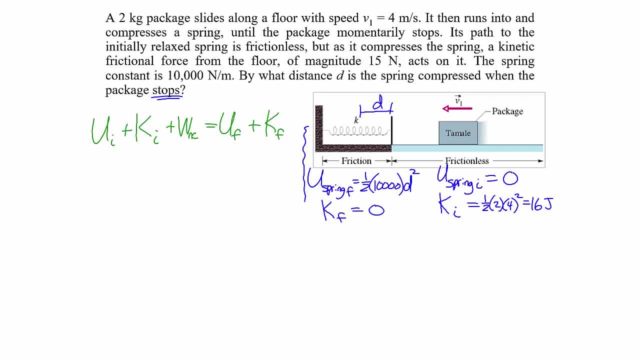 squared, or 16 joules, The final potential energy is 1 half mv squared or 16 joules. The final original potential energy that's stored in the spring is one half times the spring constant 10,000 newtons per meter times the unknown distance d squared, The final kinetic energy. 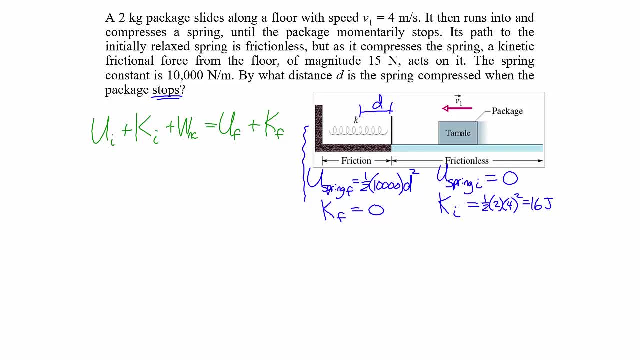 is zero, And if there was no friction, I would have just set these two things equal to each other and I could solve for d. But here there is friction. There's this force of 15 newtons that also acts over that unknown distance, d, And so the work done by that non-conservative 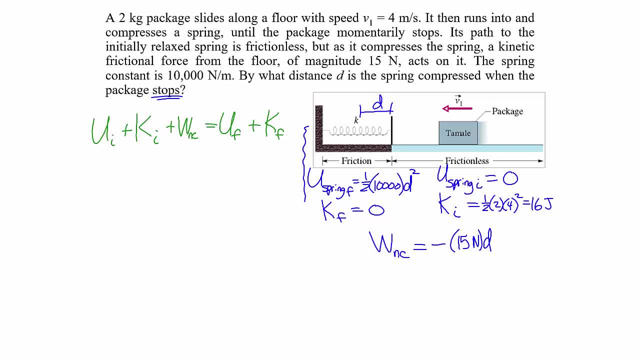 force of friction is negative because the force is opposing the motion And it's 15 newtons times that unknown distance d. So the initial potential energy of zero plus the initial kinetic energy of 16 joules, plus the work done by the non-conservative force of friction, negative: 15 newtons times d. 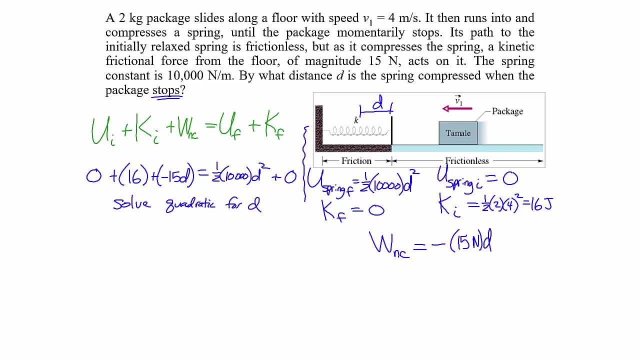 equals the final potential Potential energy one half times 10,000 newtons per meter, times d squared plus zero. And so this is a quadratic that you can solve. for d You can use the quadratic formula or you can use the solve feature if you have a TI Inspire calculator. That's what I did here. So if we use that solve, 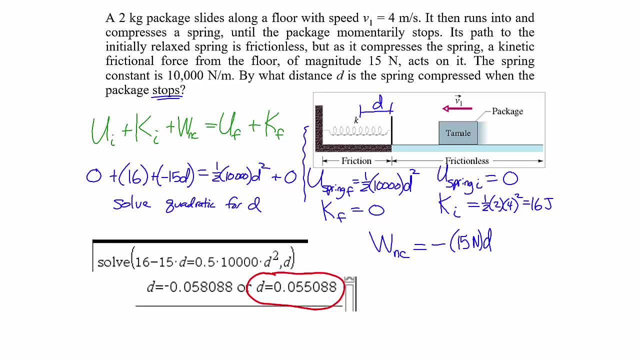 feature. it gives us that the solution to this is that the distance d is 0.05508.. Again, using the quadratic formula, it gave us two answers. If we look, we're saying that d is a positive quantity because the work done by the force of 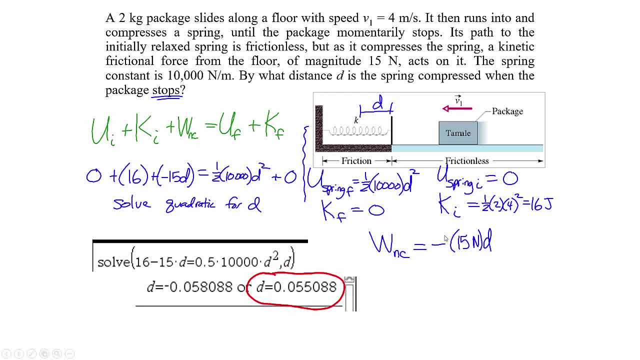 friction has to be negative. Friction is taking energy away, And so the only way that that's true is if d is a positive quantity. That's why we're throwing out the negative root and we're just choosing the positive root. This final example is just a little bit more complicated, but it's still. 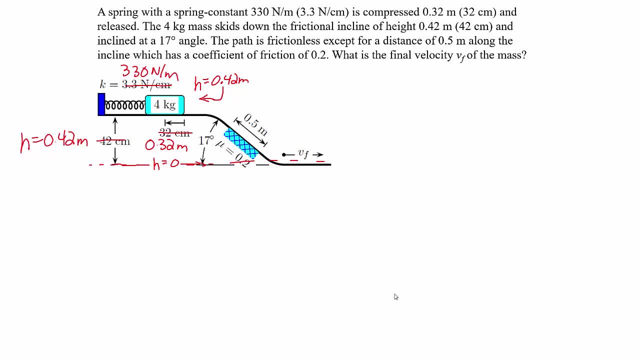 the same ideas. The thing that makes this a little bit more complicated is the fact that there's two types of potential energy in this situation. We have a spring, and so we have spring potential energy, But then we also have the height changing. 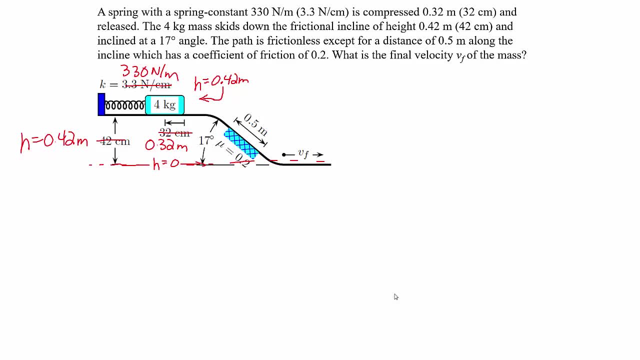 so we have a change in gravitational potential energy as well, And when you have cases like that, then the potential energy that you include in your equations is the total potential energy. It's the gravitational potential energy plus the spring potential energy at the beginning or at the 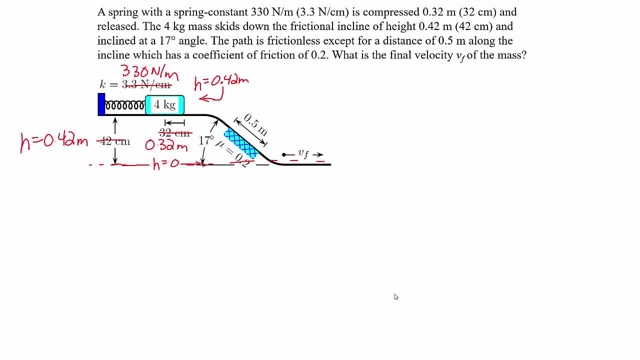 end or at some point in the middle, You include all of the types of potential energy in your equation. So here we have a spring with a spring constant of 330 newtons per meter. Again, you can see in the diagram it was given as newtons per centimeter. We need that in newtons per meter. 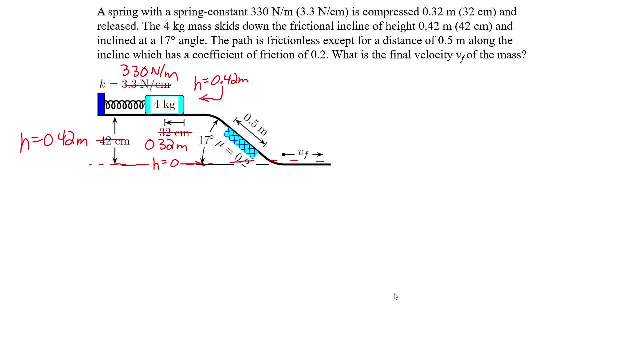 We have a four kilogram block that's connected to that spring. The spring is compressed by 32 centimeters. Again, we need to convert that to meters, so that's 0.32 meters And it's starting at a height of 42 centimeters. Again, convert that to meters, so starting at a height of 0.42 meters. 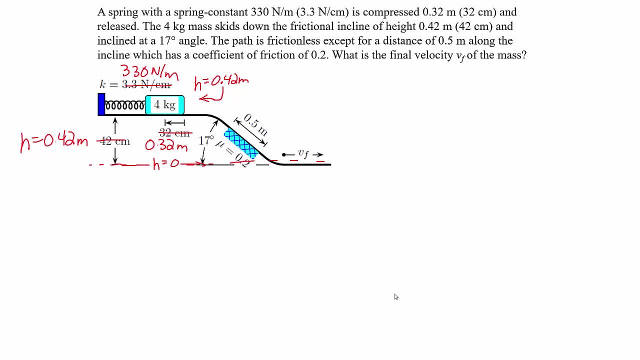 The block is pushed up again and we have a spring with a spring constant of 330 newtons per meter. The block is pushed up against the spring and released. So the block is going to leave the spring and then slide down this incline. It's a 17 degree incline that has a rough patch that's 0.5 meters. 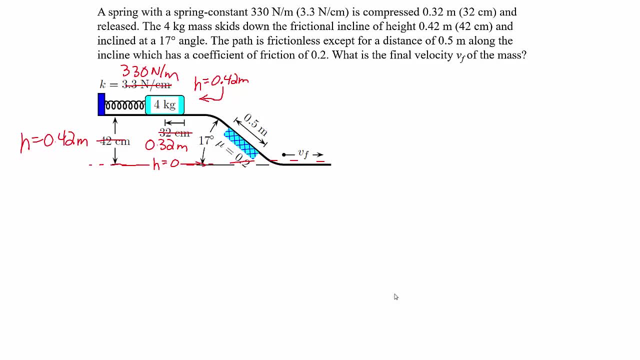 long where the coefficient of kinetic friction is 0.2.. So it slides down that rough patch and reaches the bottom of the ramp. We want to find the speed of the mass at the bottom of the ramp, And so our general form of conservation of energy says that the potential energy 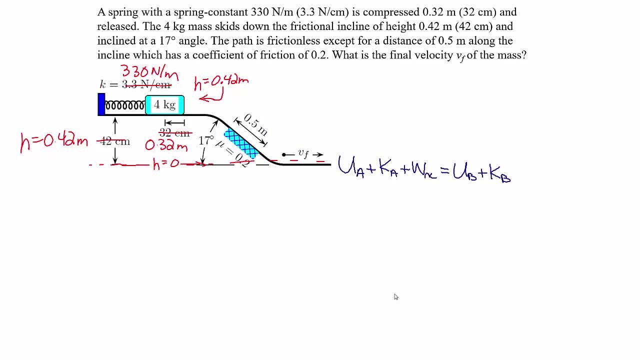 at point A plus the kinetic energy at point A, plus the work done by the non-conservative forces, equals the potential energy at point B plus the kinetic energy at point B. The potential energy at point A is the spring potential energy plus the gravitational. 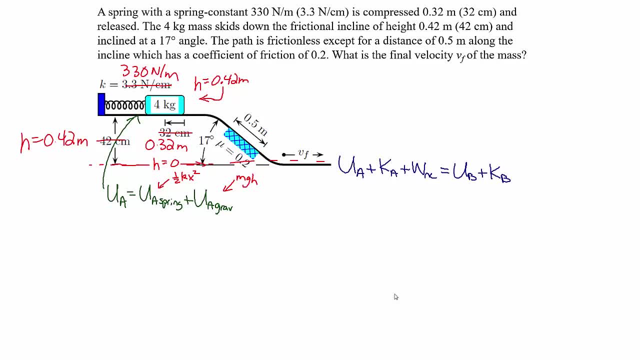 potential energy We're picking for gravitational potential energy. I'm picking that the height is 0 at the bottom of the ramp, And so that means that it's starting at a height of 0.42 meters. So we have spring potential energy plus gravitational potential energy at the beginning. 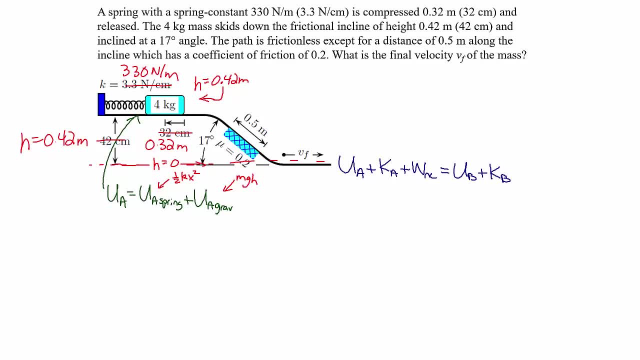 We have 1.5 kx squared plus mgh at point A. So plugging in the values, 1.5 kx squared, that's 1.5 times 330 newtons per meter, times 0.32 squared plus the gravitational potential. 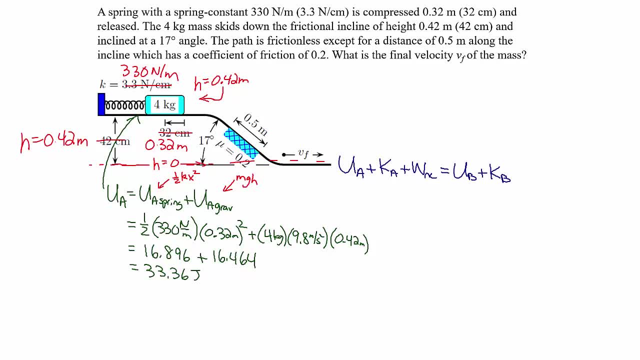 energy: mgh: 4 kilograms times 9.8 meters per second, squared times 0.42 meters, And so we had 16.896 joules of spring potential energy plus 16.464 joules of gravitational potential energy, which gives us a total potential energy at the beginning of 33.36 joules. 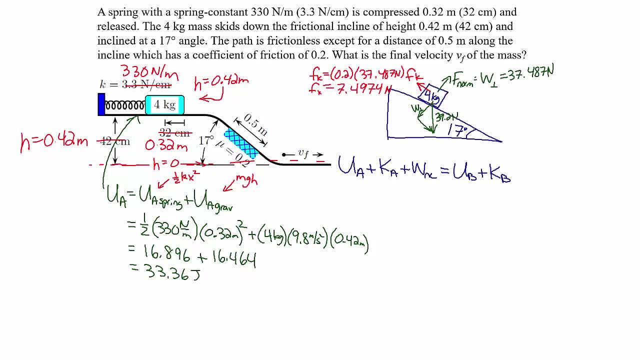 The kinetic energy at the beginning is 0. And so now we need to find the work done by the force of friction, And so the force of friction is acting on this inclined part. So I have it redrawn over here. We have this inclined. 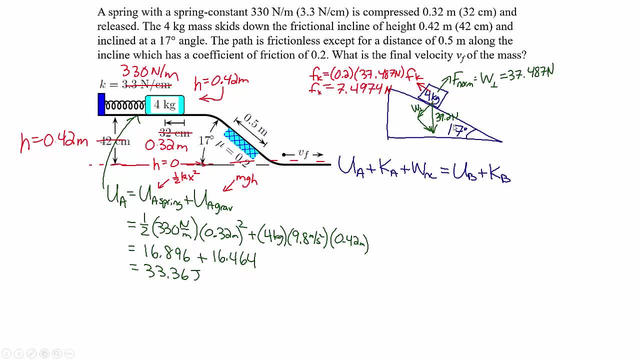 It's inclined at an angle of 17 degrees relative to the horizontal. The force of gravity on this block is 39.2 newtons. We need to know the perpendicular component of the force of gravity because that's what gives us the normal force. 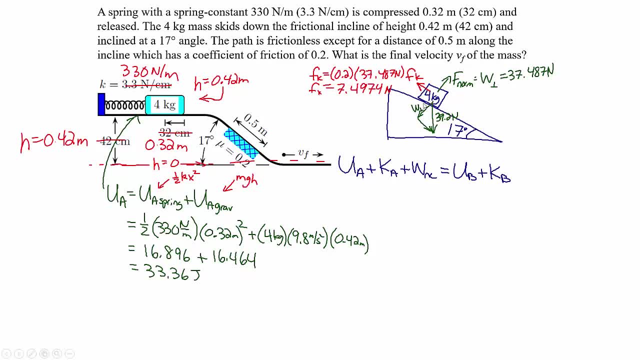 The perpendicular component of the force of gravity is the weight times the cosine of 17 degrees. So that gives us that the perpendicular component of the weight which equals the normal force is 37.2.. And so we have 17.487 newtons. 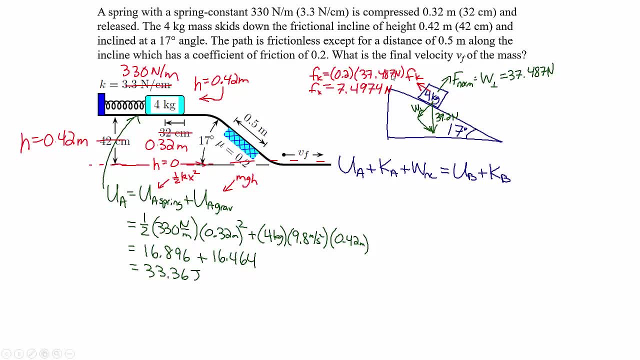 The force of friction is the coefficient of friction times the normal force. Again, it's not always coefficient of friction times the weight of the object. The force of kinetic friction is the coefficient of friction times the normal force. So here, that's why we needed to know this. 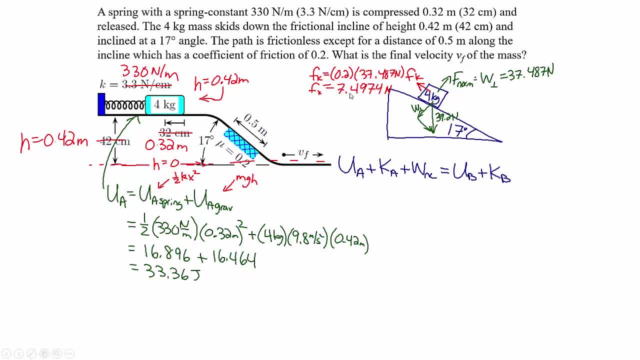 normal force. So the force of kinetic friction is 7.4974 newtons And so that force of friction is acting opposite the motion As it slides this .5 meters down the incline. So the work done by friction is going to be negative, since the force 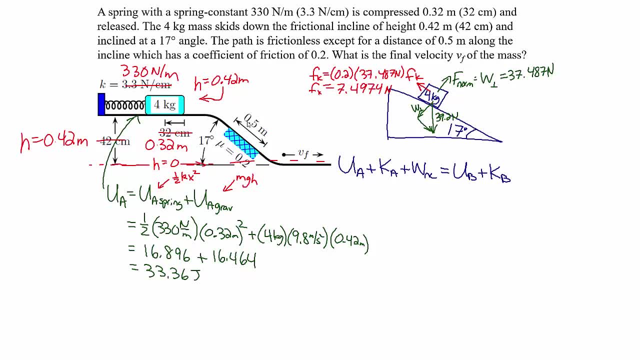 is opposing the motion, It's the force: 7.4974 newtons times the distance of .5 meters. So that work done by friction, that work done by the nonconservative force of friction, is negative: 3.7487 joules Friction is taking away. 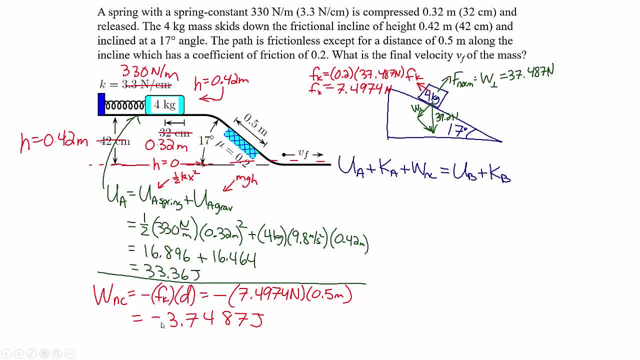 3.7487 joules. Friction is taking away 3.7487 joules. Friction is taking away 3.788 joules, 7487 joules- of mechanical energy. so anyway. so where is that energy going, that mechanical energy? 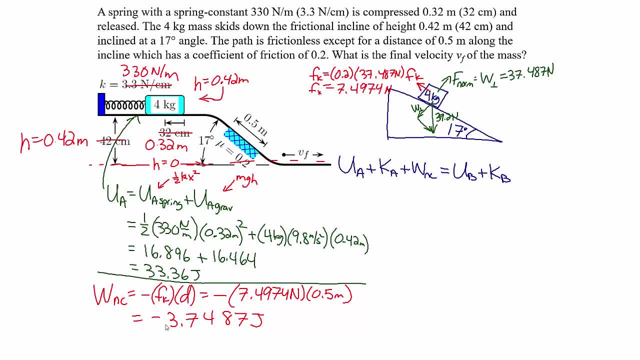 is getting converted into heat energy. as something slides across a surface, the surface heats up, but that's not mechanical energy anymore, and so we lost mechanical energy in this process. we started with 33.36 joules of mechanical energy, we lost 3.7487 joules of mechanical energy, and so that 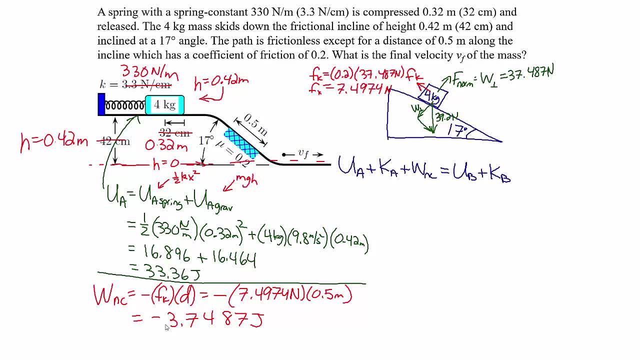 gives us what our mechanical energy is at the end when it reaches the bottom of the slide. at the bottom of the slide the potential energy is zero because the height is zero at the bottom of the slide, and so all of our mechanical energy at the end is kinetic energy. so the mechanical energy at 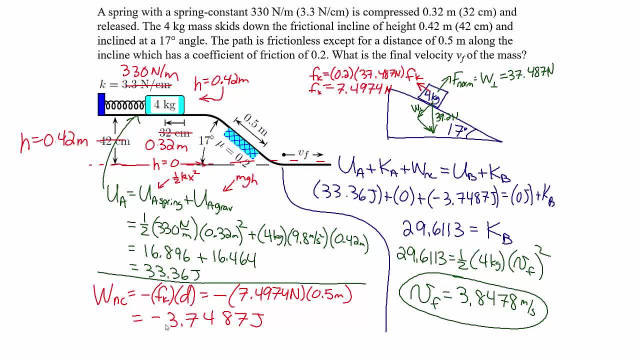 the end is 29.6113 joules, and kinetic energy is one half mv squared, and so we get that the speed at the bottom of the slide was 3.8 478 meters per second. again, this is a really good problem to put everything together, because it 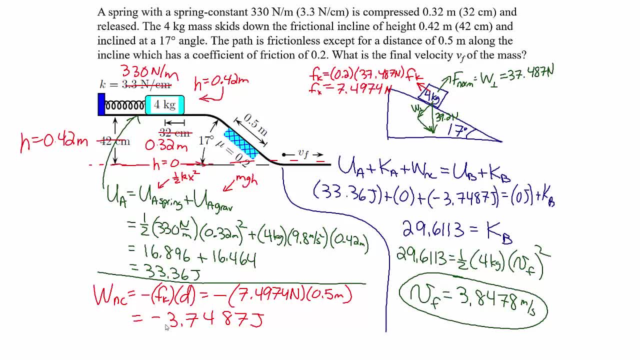 involves cases where there's more than one type of potential energy. you just include all of the types of potential energy added together when you look at your conservation of energy equation, and this also involves work done by friction and so how we include that in the equation. problems involving non-conservative forces: they're not any more. 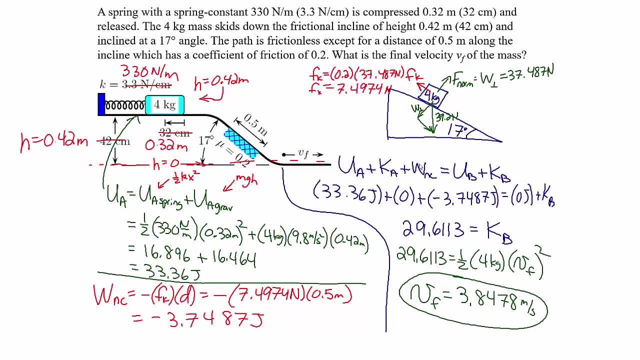 difficult to do. it's just extra things that we have to take into account. besides calculating the kinetic and potential energies, we also have to be able to calculate how much work is done by the non-conservative force, so we can include it in the equation in some later videos. there are some other.